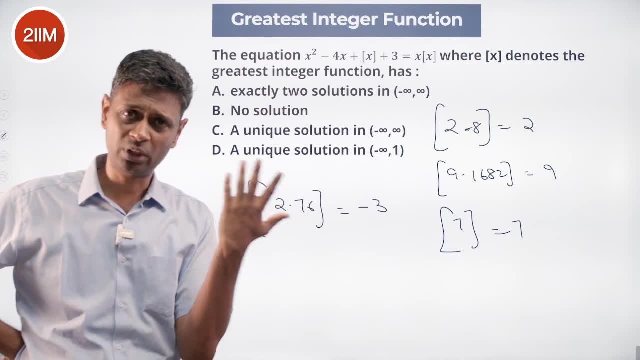 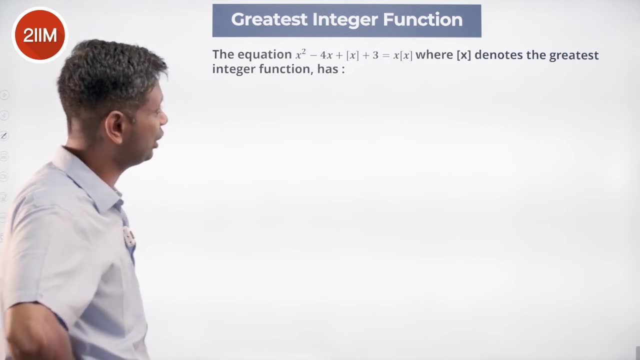 below minus 2.76 is minus 3.. That is what the answer is. So x square minus 4x plus greatest integer of x plus 3 equals x times integer of greatest integer of x. Let us see if we can simplify this. Let us bring everything to one side. 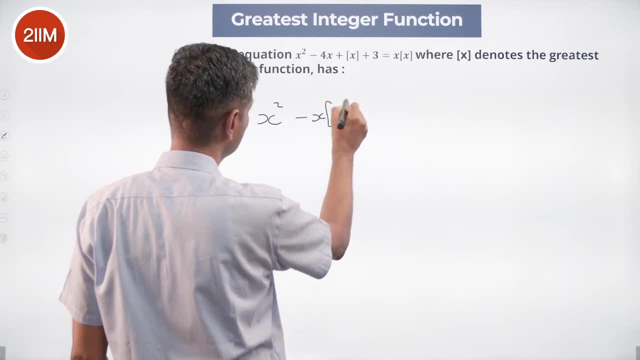 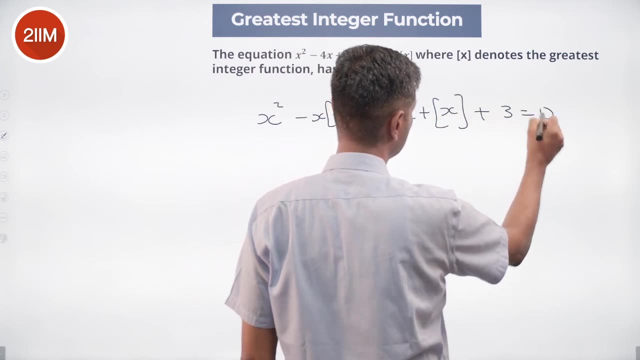 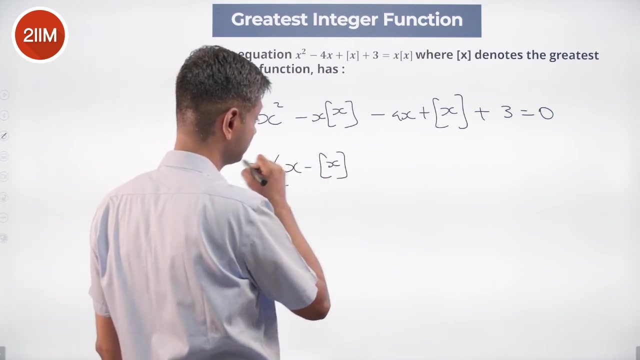 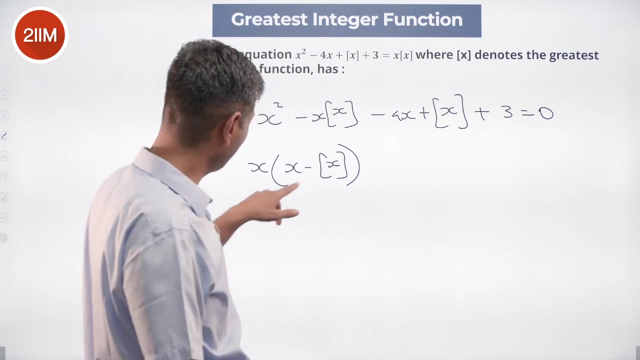 So x square minus x times greatest integer of x minus 4x plus greatest integer of x plus 3, equal to 0.. Nice, We are going to take out an x. We are going to take out x minus greatest integer of x Minus 4x plus greatest integer of x, With an x minus greatest integer of. 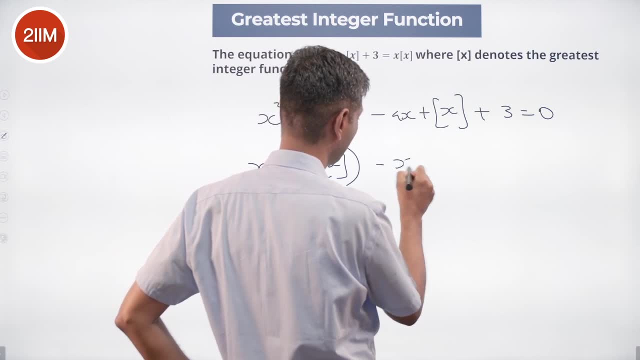 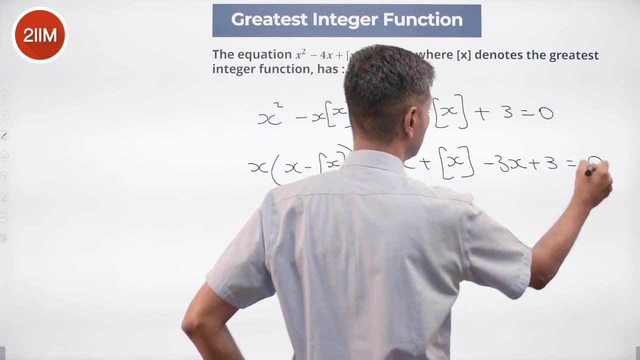 x. Let us see if we can pull this off Right. this is minus x Minus 4x, plus greatest integer of x, minus 3x plus 3, equal to 0.. Why am I doing this? This is an x minus greatest integer of x. Let us create one more x minus greatest integer. 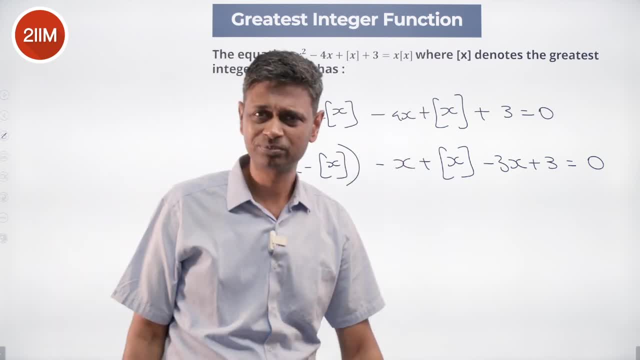 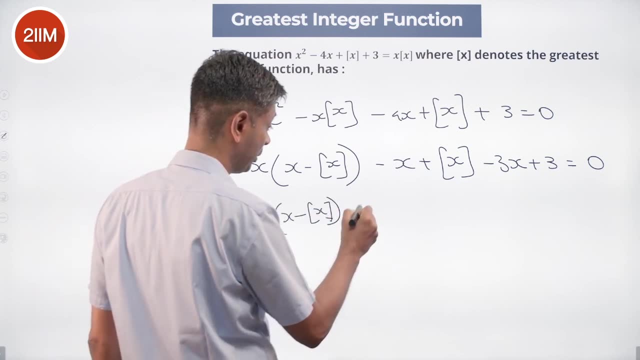 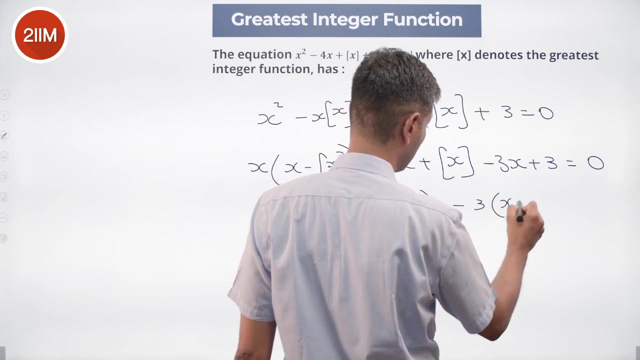 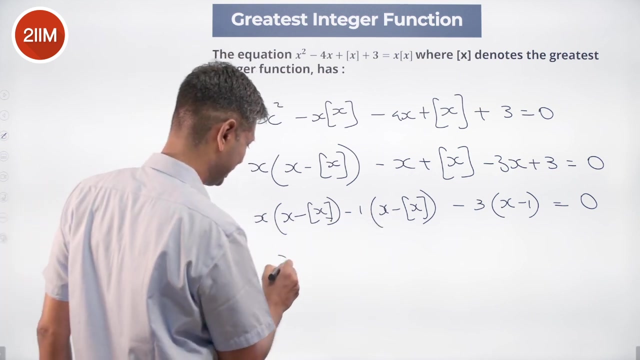 of x. So break this as minus x minus 3x. Nice, So this becomes x times x minus greatest integer of x minus 1 times x minus greatest integer of x minus 3 times x minus 3 times x minus 1, equal to 0.. This is lightly factorizable: x minus 1 times x minus greatest. 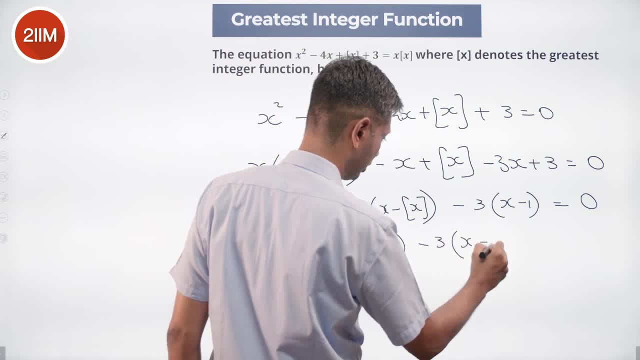 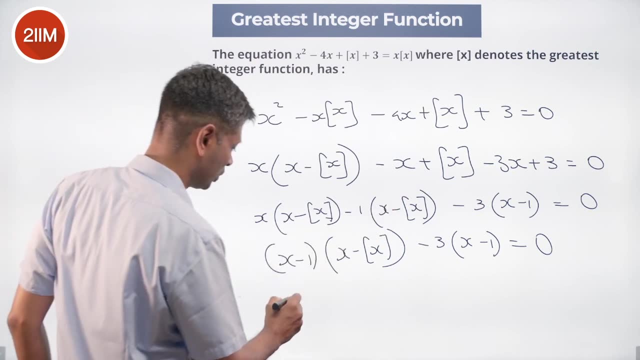 integer of x minus 3 times x minus 1 equal to 0.. Nice Again, an x minus 1 is common. Take out an x minus 1 common and say x minus 1 into x minus 1 minus 1 minus 2 x minus 1. times x minus 1 is a common. If we are going to Va alltosex of x minus x and so on, Okay, So we are going to even out all the number of 8 and every number of 8, and even out all of it, Then we will have an x plus x minus 1 times x minus 1 times x minus 1 equals. 0 and the delta, and even add all that together. So let us bring everything to one side, and it should beidelсят here. If it is spooning that the above and below a of x minus 1, then it is possible that 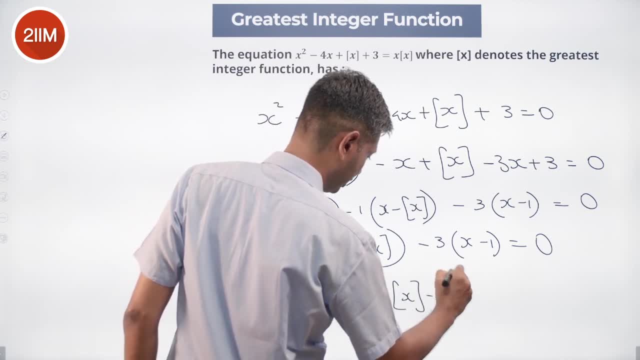 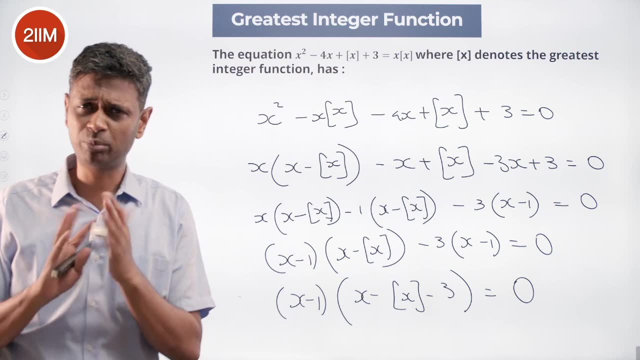 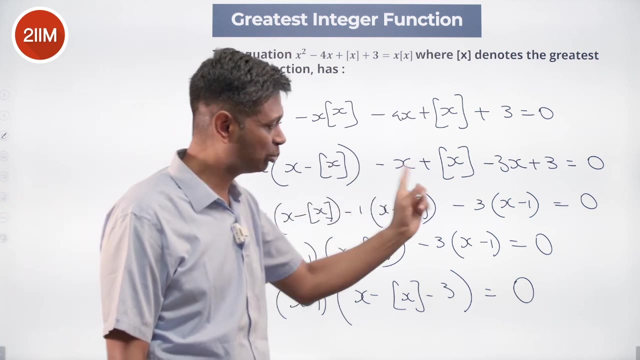 minus greatest integer of x minus 3, equal to 0. Nice, brilliant. So we have nicely factorized this rather brilliantly, And so bring this to the side. there is an x minus greatest integer of x. we want to contrive another x minus greatest integer of x. put that in. 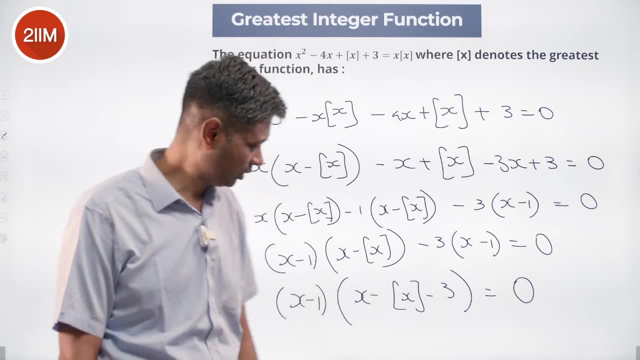 remaining is minus 3. x plus 3,. stick it in the end, get through. And so now, x minus 1, when will it go to 0, when x is 1?? So x equal to 1 is our solution. 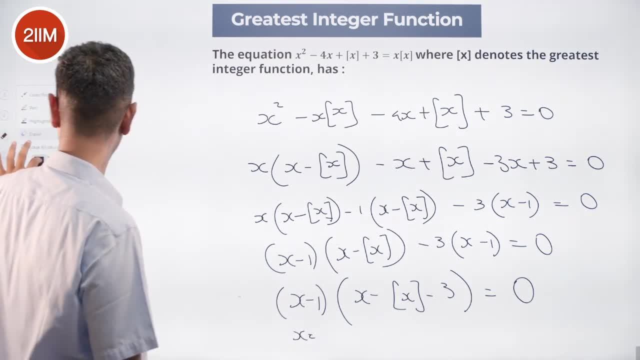 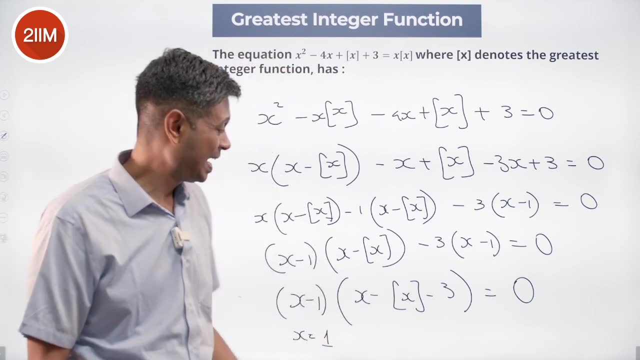 x equal to 0, x equal to 1 is our solution. x minus 1 equal to 0, x equal to 1 is our solution. Nice, x minus greatest integer of x minus 3, when will it go to 0?? x. greatest integer of x is the. 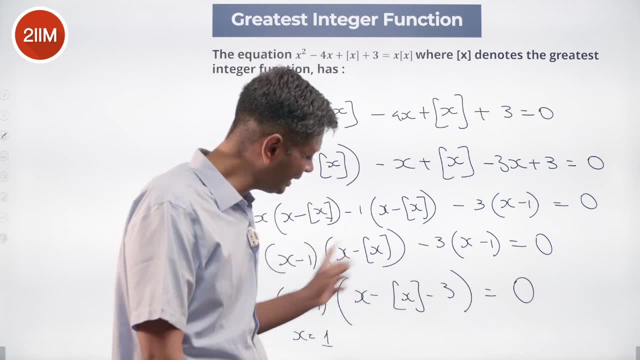 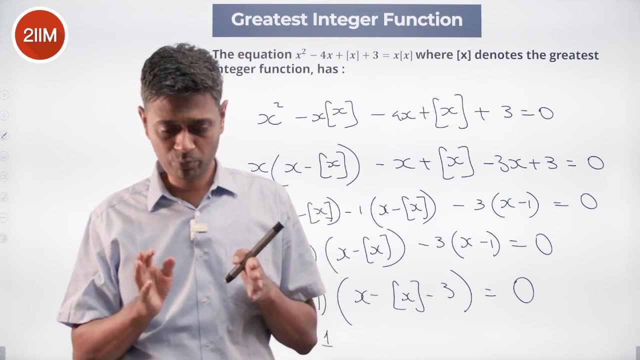 greatest integer less than or equal to x. x minus greatest integer of x cannot be more than 1.. Anything from 3 to 4 will be written as 3, 3.3 to 3.999999,. greatest integer of that is 3.. 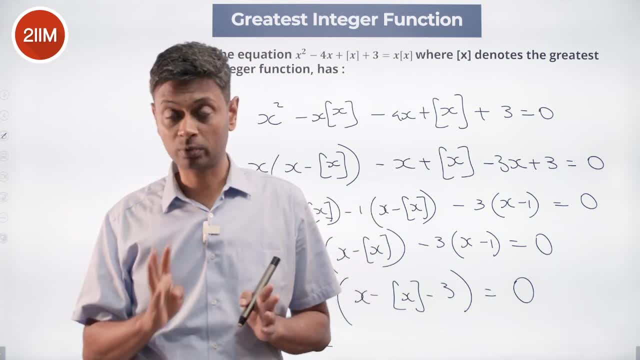 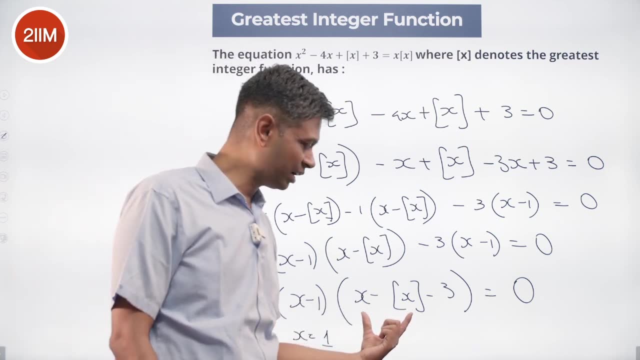 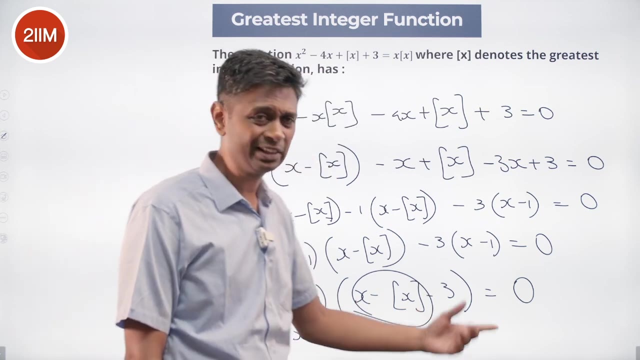 4 to 4.999999,. greatest integer of that is 3.. integer of that is 4.. x minus greatest integer of x cannot be 1 or more. This x minus greatest integer of x, this part, is less than 1.. A number less than 1 minus 3 cannot go to 0. So this part. 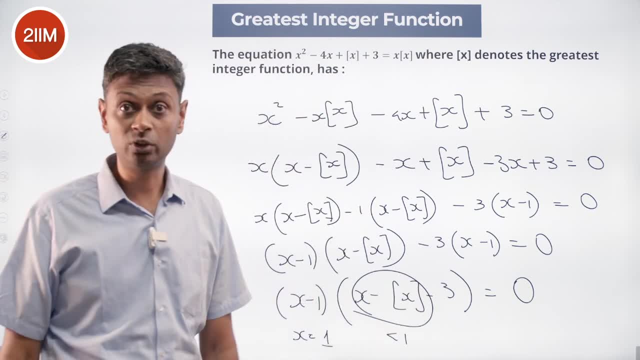 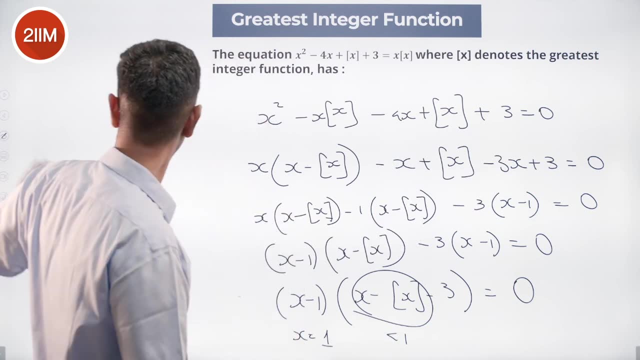 cannot go to 0 at all. This can go to 0 at x equal to 1, or x equal to 1 is the one solution and only solution for this. Nice So, x equal to 1,. let us look at the choices. 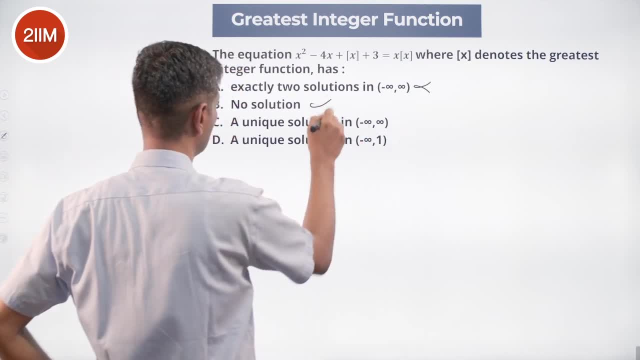 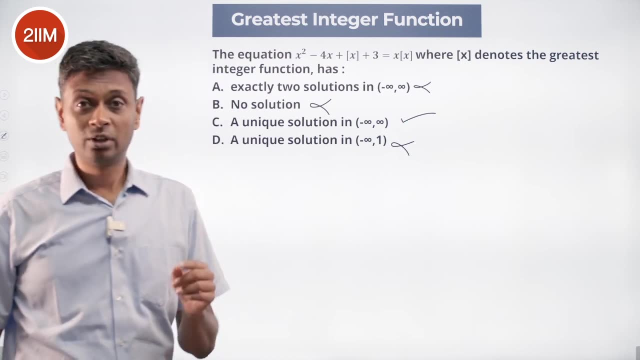 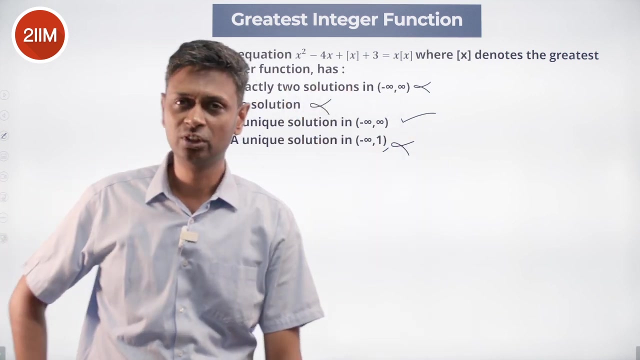 Exactly two solutions. no, No solution. no. A unique solution in minus infinity: yes, Unique solution in minus infinity to 1, no, This does not include 1.. So there is only one solution: x equal to 1 works, Nothing else works. So there is one solution in the range of minus. 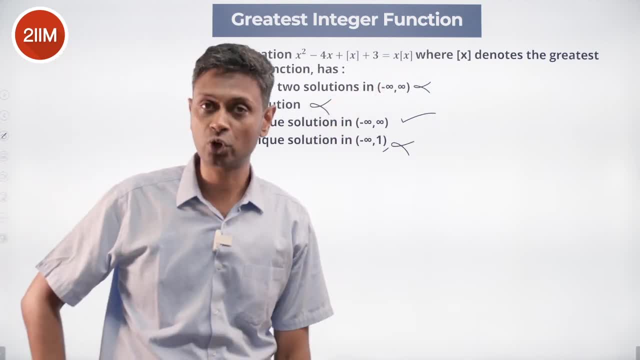 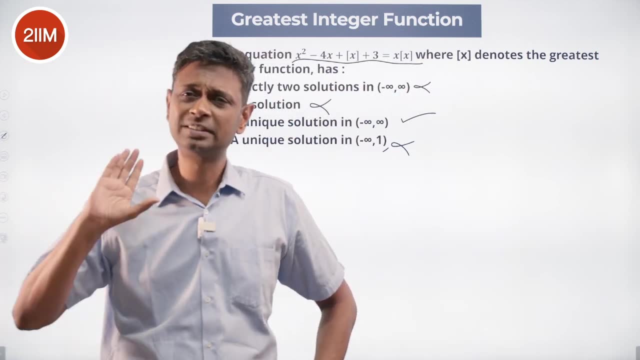 infinity, to infinity. None of these work. And the choice C, C for chocolate. This is actually beautifully factorizing. And the rule of thumb: whenever you are looking to break something down, bring everything to one side, stick it to 0 and see there is some way of manipulating it. 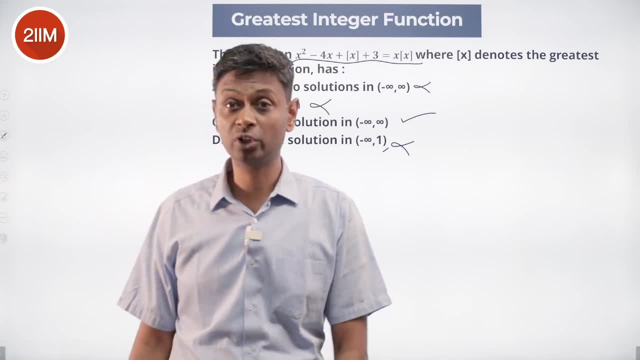 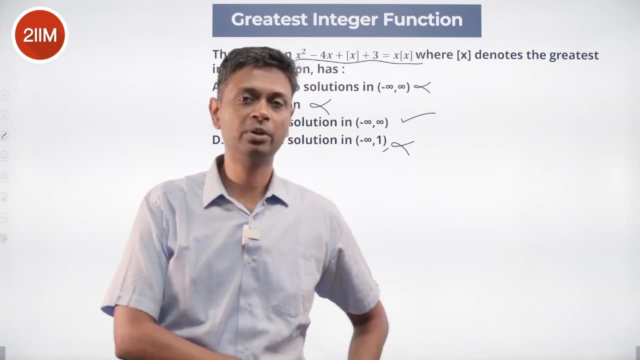 factorizing it. to simplify it, It factorizes rather beautifully as x minus 1 into x minus greatest integer of x minus 3.. x minus greatest integer of x minus 3 cannot go to 0.. x minus 1 goes to 0 and x is 1.. Then we simplify this. 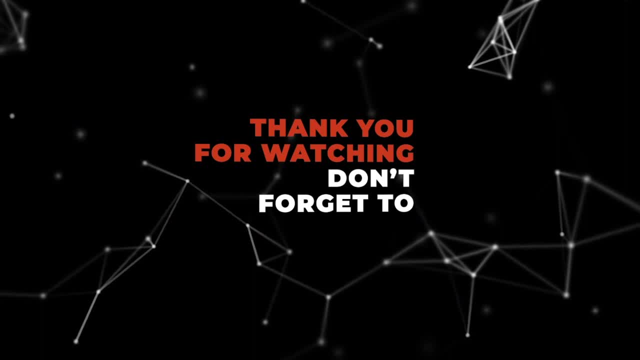 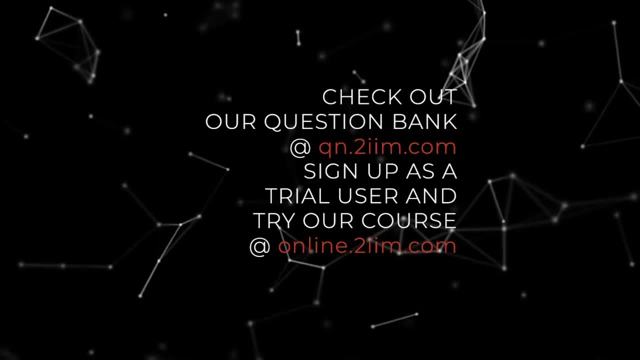 And we solve this with minus infinity as minus infinity. And that is it for this video. friends, Thank you very much, And may God bless you all.